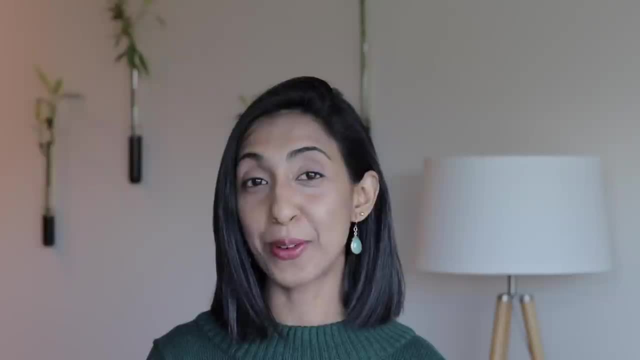 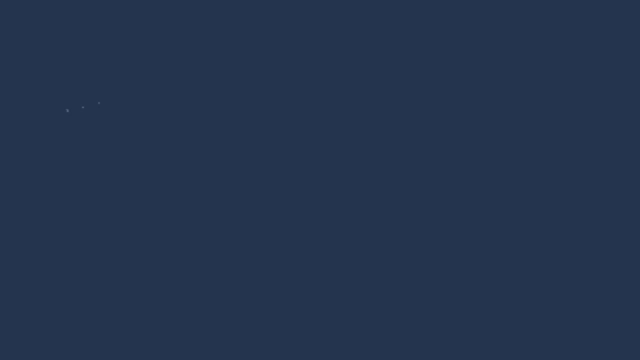 art like painting and graphic design, and framing it in a way that makes sense for what we do as designers, when we're using our design software to choose colors and make them look good together. This is my super practical, non-technical guide to color palettes and color theory in UI design. 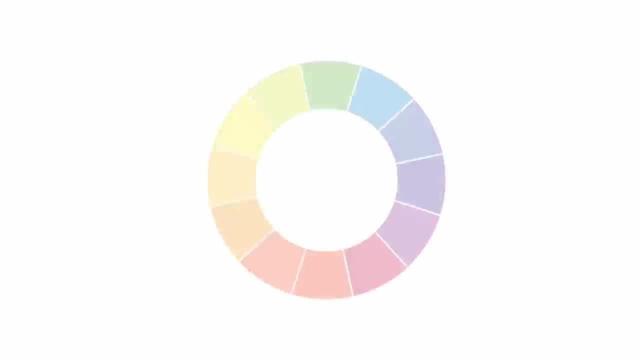 So you followed all of the color harmony and color theory tutorials to a tee and generated a complementary color palette. But you noticed that the colors don't seem to match very well or don't look great on your UIs. Perhaps they look harsh or are a bit muddy and unprofessional and you don't really know why. 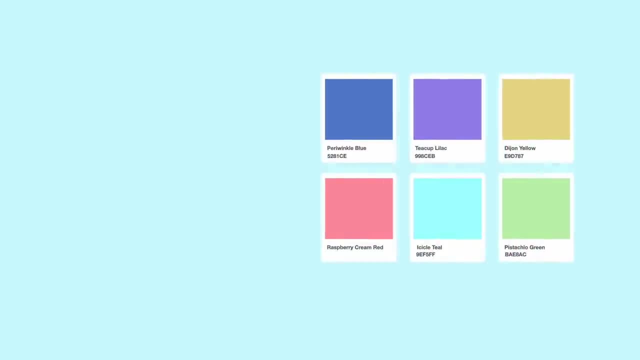 What do you do now? Color harmony and color theory offer some formulas that we can use to start our color palettes. It's an important foundation to understand and I've done a video all about color harmony and color theory here on our channel. 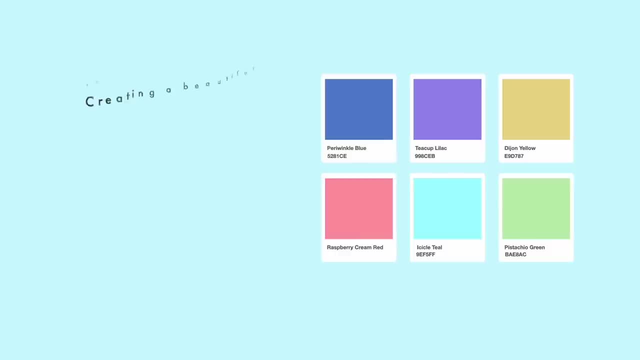 But creating beautiful color palettes isn't only about these formulas. It's also about subtleties, of balancing hue, tint, tone, shade and temperature. These are the levers that we can push and pull to achieve more balanced and unique color combinations. 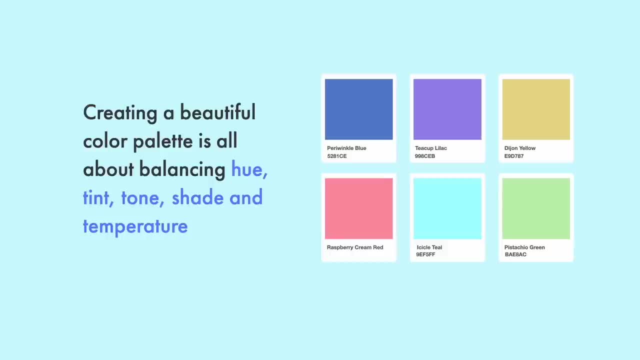 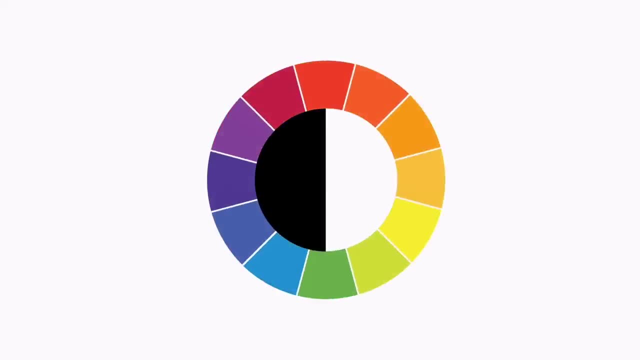 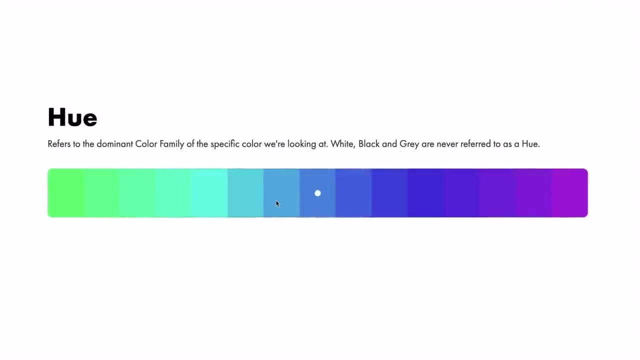 for our UI designs. So first a little refresher on what these levers are and what they do. A hue refers to the dominant color family of the specific color we're looking at. White, black and gray are not usually referred to as hue or color. 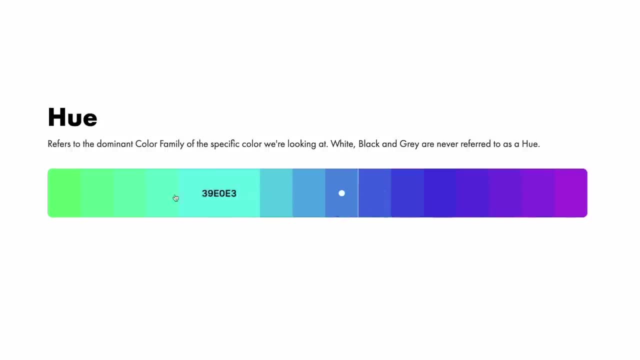 A tint is any hue or mixture of pure colors with only white added. A tint lightens the color, but it doesn't make it brighter. Therefore, a tint can range from slightly lighter to a little bit lighter. A tint can also be used to add color to your design. 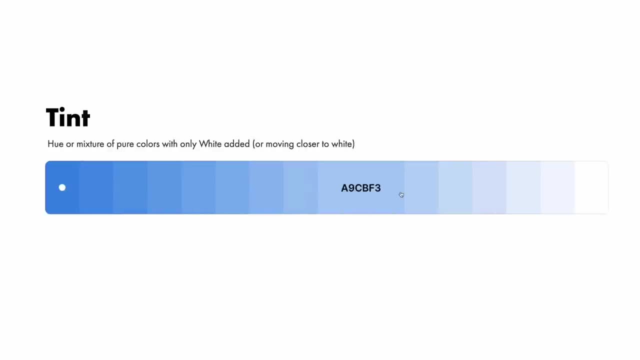 A tint can range from slightly lighter than your original color all the way to white with barely any of the color mixed in. In our color pickers this means moving closer to white Tone is any hue or mixture of pure colors with only gray added. 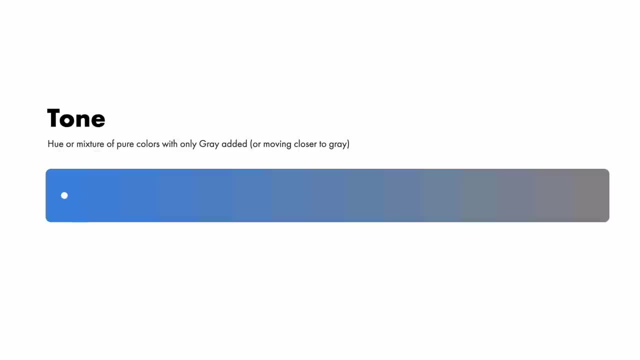 or moving closer to gray in our color pickers. To be precise, the definition considers gray as truly neutral. In other words, there are no pigments in the gray and black, A neutral mixture of gray, no matter how light or dark. 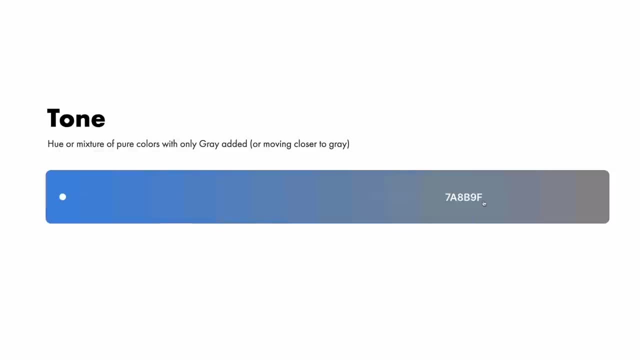 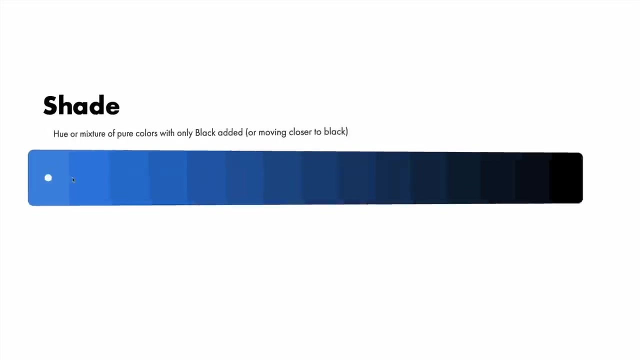 will tone down the intensity of any color. Tone colors are generally considered more pleasing to the eye. They are complex, subtle and sophisticated. That's because bright, pure colors are more often associated with children and primary colors. Shade is any pure hue or mixture of pure colors with only black added. In other words, it contains 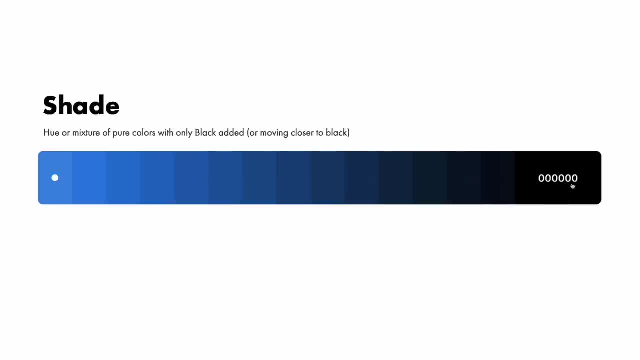 absolutely no white or gray. A shade darkens the color. It remains the same hue, only a darker version of it. Therefore, a shade can range from slightly darker than your original color all the way to nearly black, with barely any of the color mixed in. 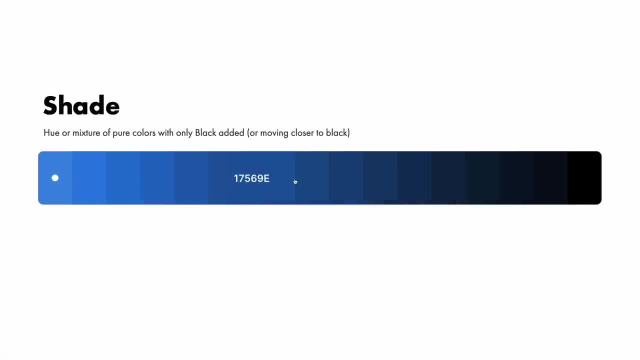 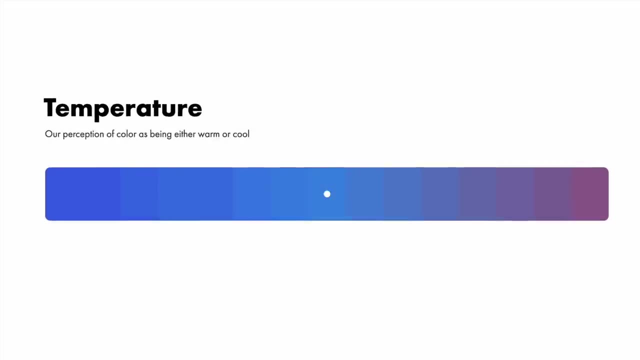 Done by adding a touch of black to your color or moving your color picker closer to black. Temperature is more about how we perceive the hue that we're seeing, And we tend to divide these into two categories: warm or cool. Warm colors are the colors that come from. 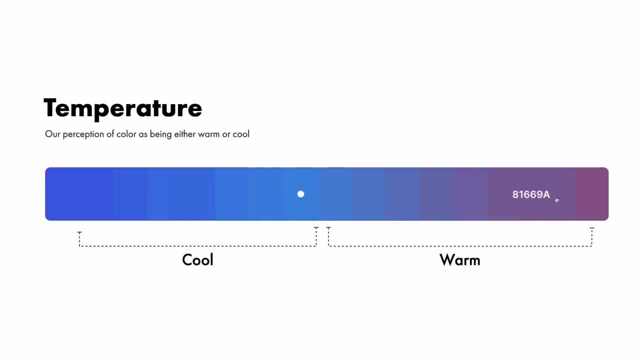 increasing the red or yellow tones in a hue. These tend to evoke the feelings of passion, coziness, energy and motion. They remind us of sunlight and heat and are often referred to as active colors. Cool colors are the colors formed from increasing the blues and greens. These tend to invoke 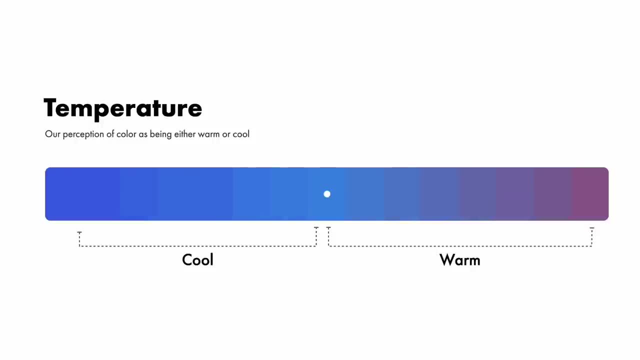 freshness, warmness and coolness. Cool colors are the colors formed from increasing the blues and greens. These tend to invoke freshness, warmness and coolness, Winter stillness and calming. They remind us of ice, snow and water and tend to be considered passive colors. 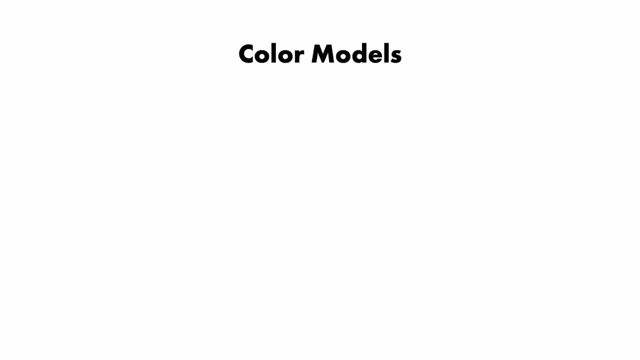 To start off, it's important to understand what I mean when I refer to adding white, black or gray, Since we're not working with paint and we're not actually mixing physical colors together when we design UIs. we need to think about this in terms of screens And for that. 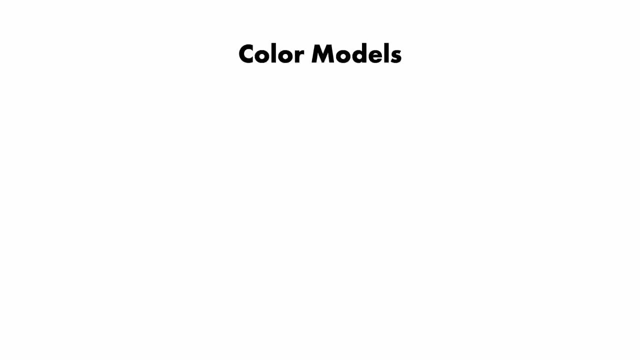 we're talking about light And the mixing of that light. To get a little technical, there are three different color models you may have heard of. that will help us understand how light and color work together a little better. The first is CMYK, which stands for 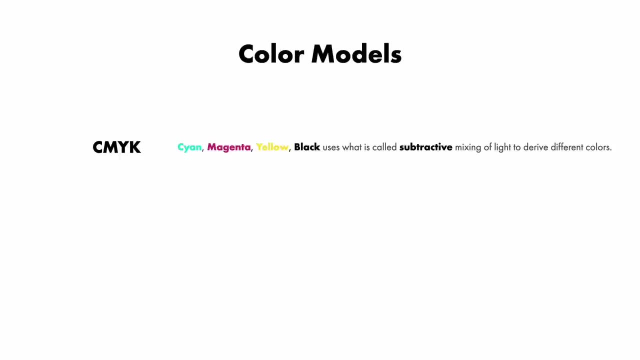 Cayenne, Magenta, Yellow, Black. This uses what is called a subtractive mixing of light to derive different colors. RGB stands for red, blue and green, and uses what is called additive mixing of light to derive different colors. And finally HSB, or sometimes the B is. 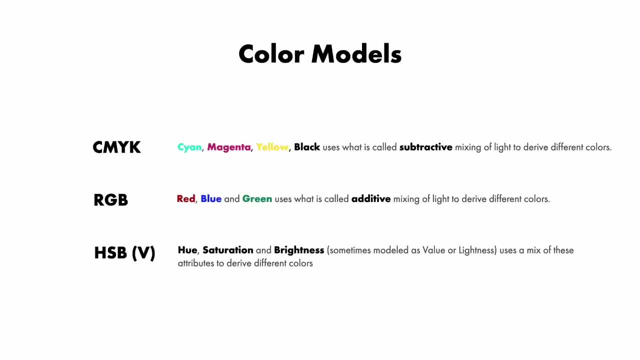 referred to as V for value stands for hue, saturation and brightness. This uses a mix of these attributes to derive different colors. CMYK is called subtractive because it refers to the light and the page, Because a page doesn't project light or shine it at us. the page has to reflect light off of it. 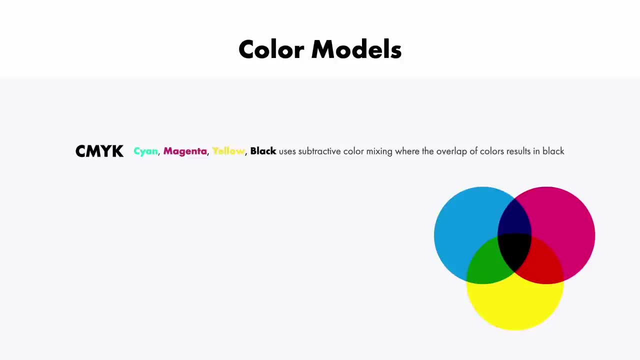 So when mixing these colors together, you are in effect covering up the white of the page and thus reducing the amount of light that is able to be reflected off of it. Kind of like a kid mixing all of the finger paint colors together and getting black. CMYK color models are mostly used for pages and with printers. 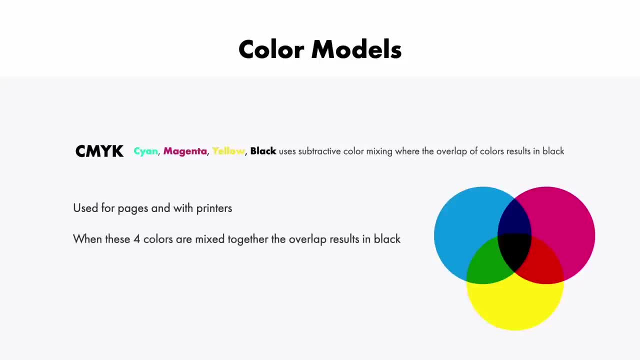 When these four colors are mixed together, they are called subtractive. When they are mixed together, the overlap results in black. Subtractive means you are removing the white that's there or covering it up on the page. RGB is when red, blue and green light is mixed together and the screen shines and 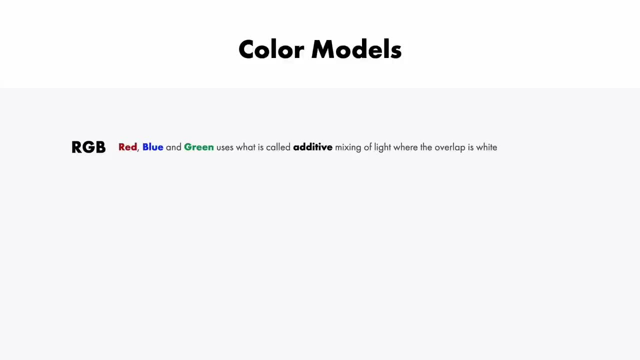 projects that light out at us. The overlap of all of these colors at full brightness results in us seeing white, Kind of like being blinded by bright floodlights. RGB color model is used for digital screen design. It's like having three bright red, green and blue lights projecting out at us at full brightness. 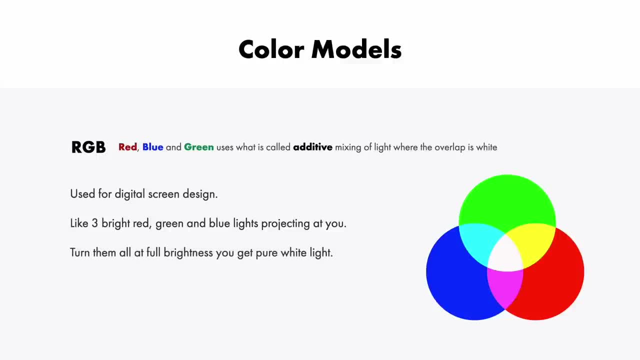 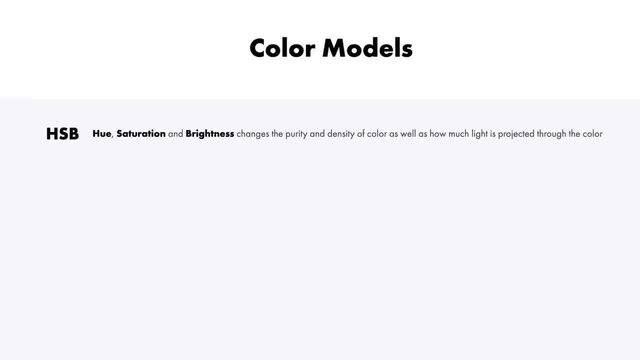 Turn them all on and you get pure white light. Turn them all off and you would see blackness. Finally, we have HSB Hue, Saturation and Brightness. These values change the purity of the colors that are projected out at us. These values are: 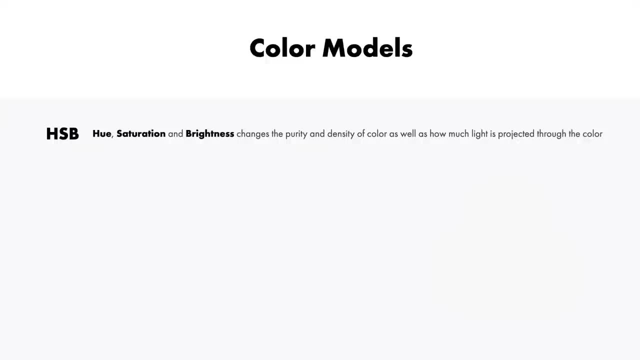 used to change the purity and density of color, as well as how much light is projected through that color. Most of you might be familiar with this, as it's what we most commonly see in our design apps as UI, UX and product designers. The HSB color model provides us. 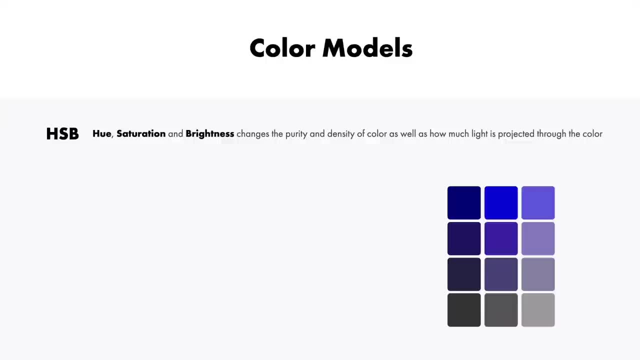 with a radial of color or a color wheel in which we have a range of hues, which are the colors, saturation, which is how much of the color there is, and brightness, how close to white or black on the screen. When we're done with that, we can go to the next slide. 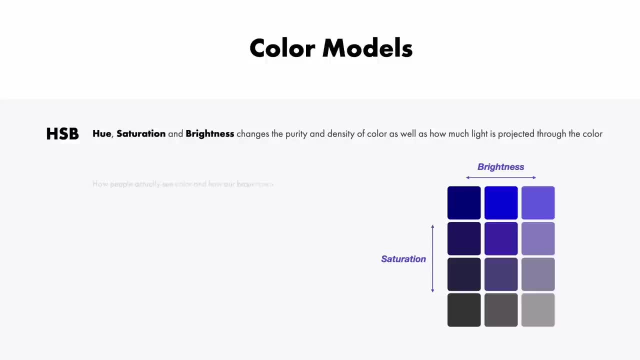 black on the scale. the value is: This is how we actually see color and how our brains work. It's most commonly used by UI and visual screen designers. The hue is represented on a radial 360 degree scale. of all colors, The saturation is: 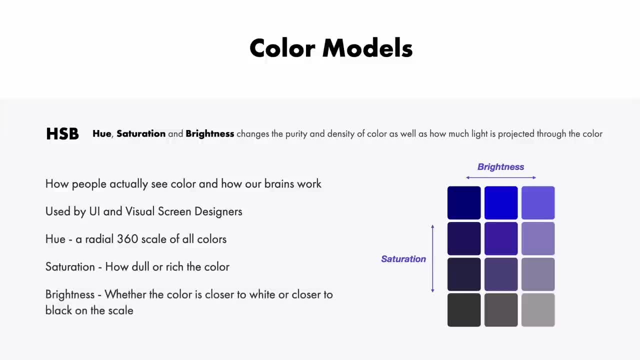 how dull or rich the color is and the brightness is whether the color is closer to white or closer to black on the scale. By mixing the hue or color from the color wheel with the saturation and the brightness would result in a specific color. So, for the purposes of this lesson and choosing colors for our 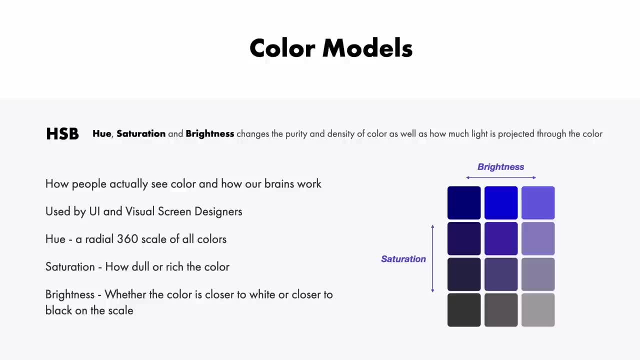 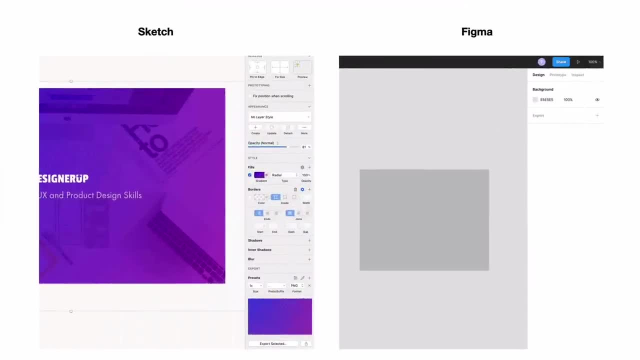 UI designs and in screen work we are going to be using this color model. Now the computer doesn't know if you're designing for screen or paper and therefore it must be told by our design apps By default. the computer will not know if you're designing for screen or paper. 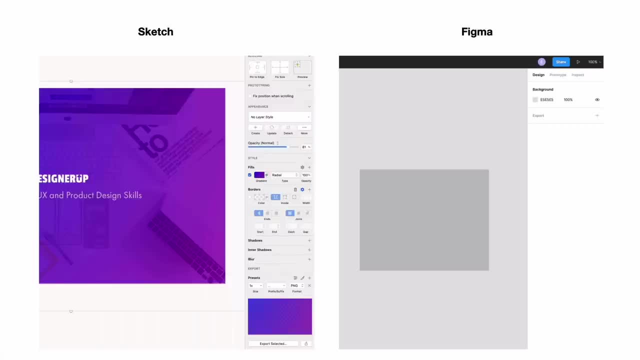 By default. the computer will not know if you're designing for screen or paper. By default, design programs like Sketch and Figma might show RGB for screens, but you can easily change this to HSB in your design app. Just keep in mind that. 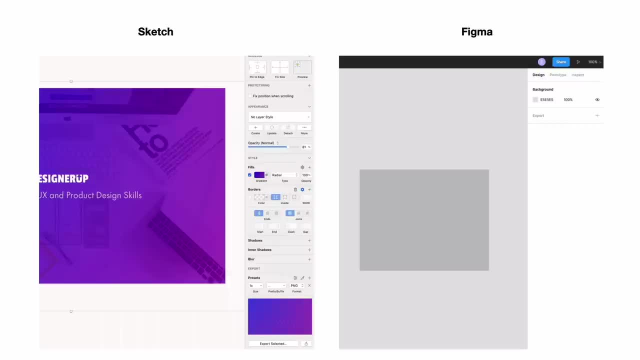 if you are changing to CMYK. not all colors are CMYK and RGB reciprocal. As I mentioned for this video, we're going to focus on the HSB color model for our world of digital UI screen design, So the first thing you'll need to do is switch your color model or color. 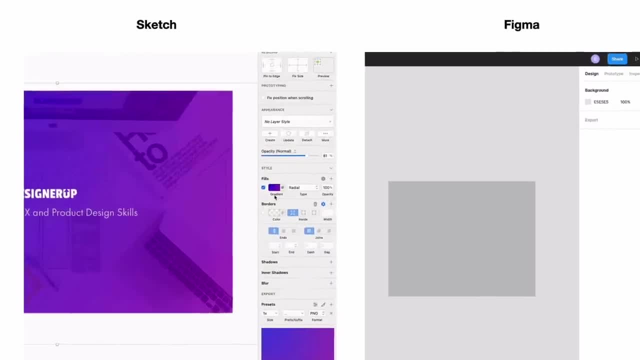 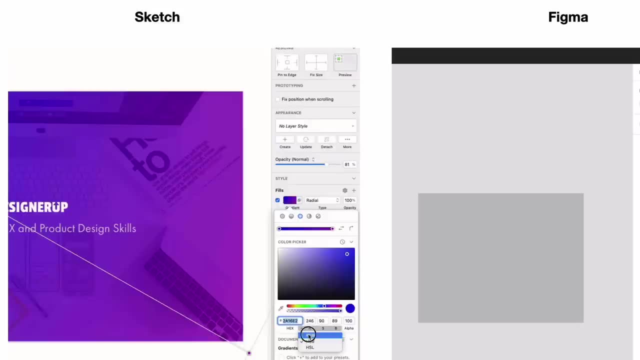 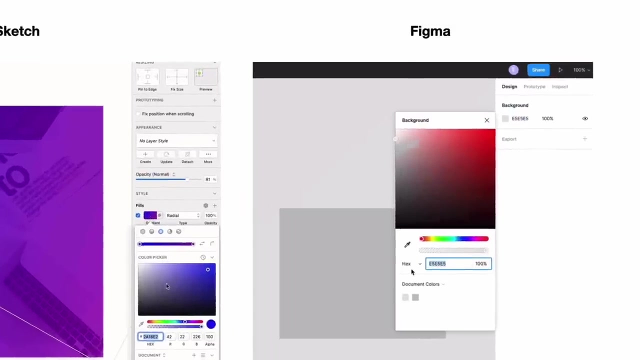 space in your design app For Sketch. you can find that by clicking on a fill and looking for the drop-down. that's next to the hex, and you should be able to toggle between the different color models. So go ahead and select HSB In Figma, it's just as easy. Click on the color swatch and click on hex to toggle. 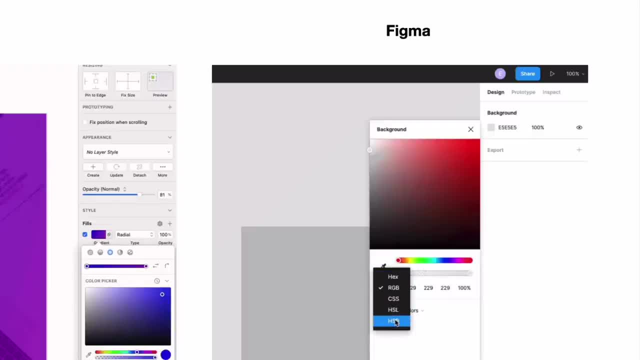 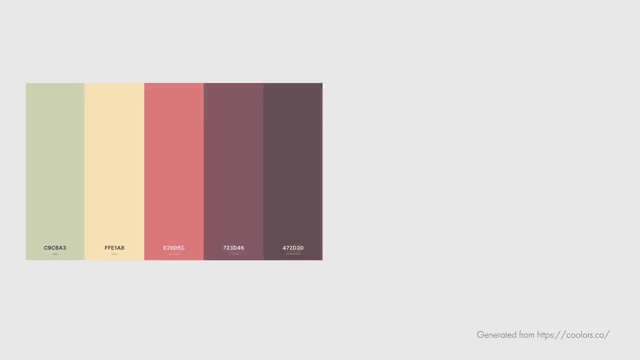 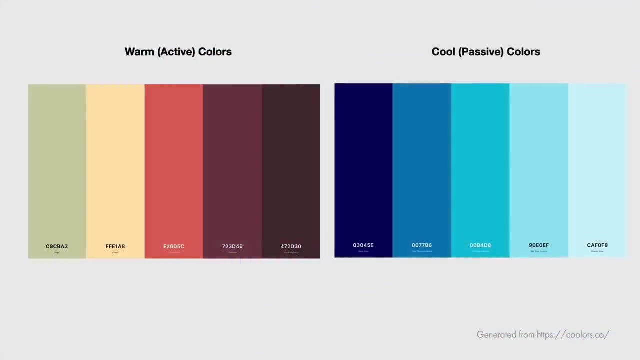 between the different color spaces. Just select the color space and click on the hex. In Figma you decide which color. In F Initiative you are simply going to be selecting HSB. There are two large groupings of colors that you often hear about- warm and 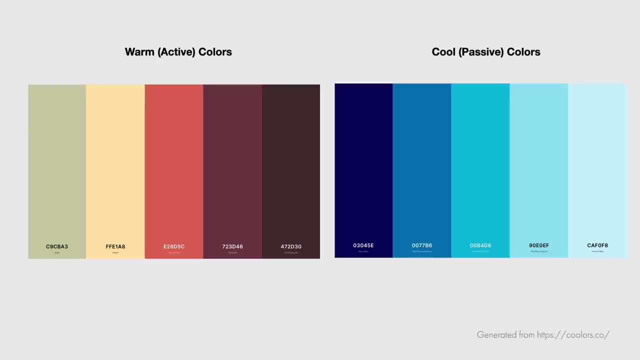 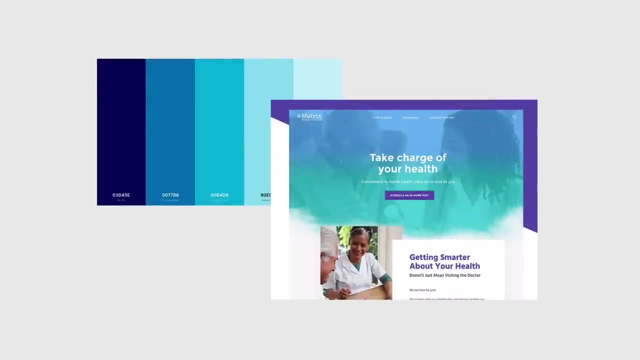 cool, Warm colors are often considered active colors because they draw more focal, while more vivid colors play an active role In UI design. we talk about visual hierarchy and primary and secondary colors. Both warm and cool colors can act as primary or secondary colors, depending on the brand focus. 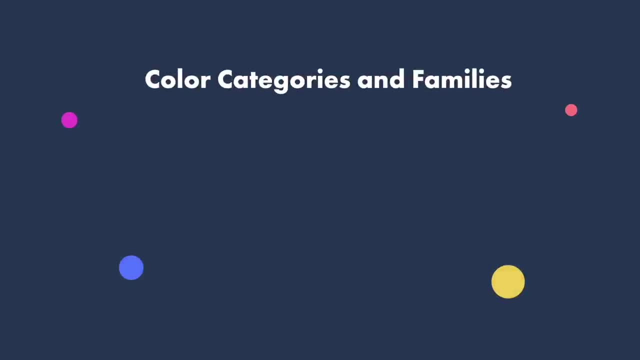 So now that you understand how colors appear on screen and on paper and all the ways we can adjust them, let's talk about how we can pull and push on these levers in our design software and balance our color schemes and color palettes. But I'm going to talk about it a little bit more like a painter or an artist to help make this all a little less technical and a little more practical and relatable. 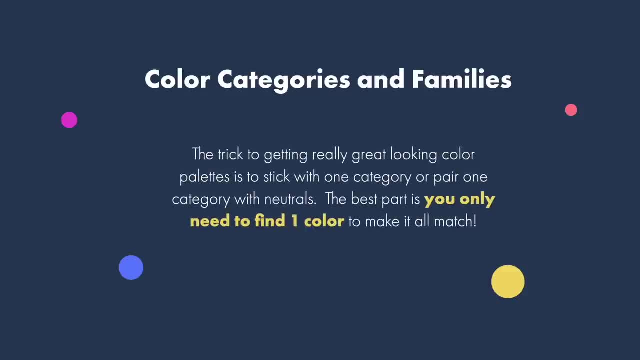 The trick to getting really great looking color palettes is to stick with one of the following categories or pair one category with neutrals. The best part is you only. You only need to find one color in your palette to make all of the rest match. 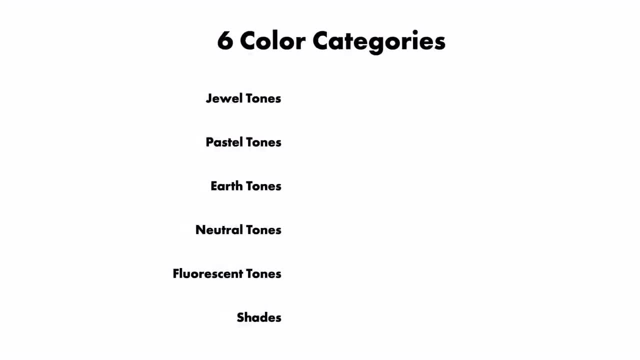 In order to derive these different color categories, we'll be focusing on pushing and pulling the levers of hue, saturation and brightness On digital screens. I've discovered that there's a formula and a safe range of saturation and brightness for each one of these, following six color categories. 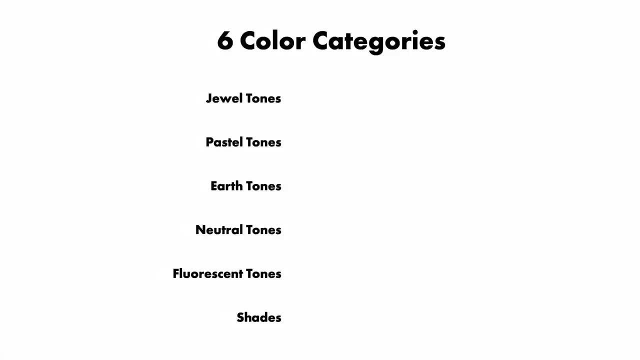 that will result in a perfect palette for every category every time. But in order to really get this all into play, we're going to need a palette that is well-tuned and well-balanced. The first category is jewel tones. The second is pastel tones. 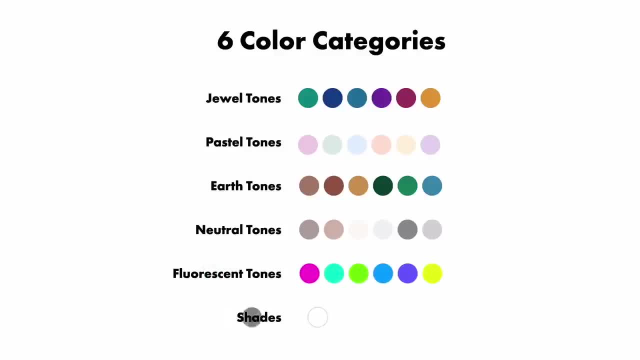 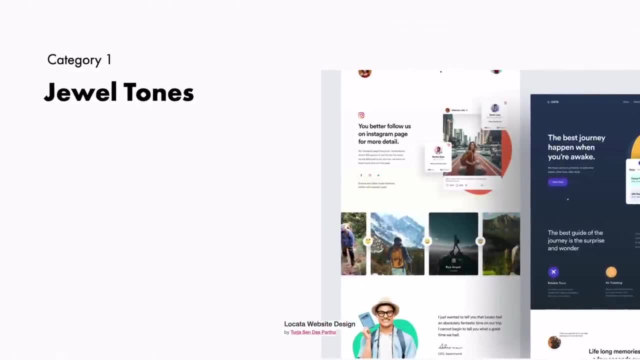 Category three is earth tone. Category four is neutral tones. Category five is fluorescent tones And, finally, category six are the shades. Category one: jewel tones. These colors are richly saturated hues named after gems like sapphire blue. The first category is jewel tones. 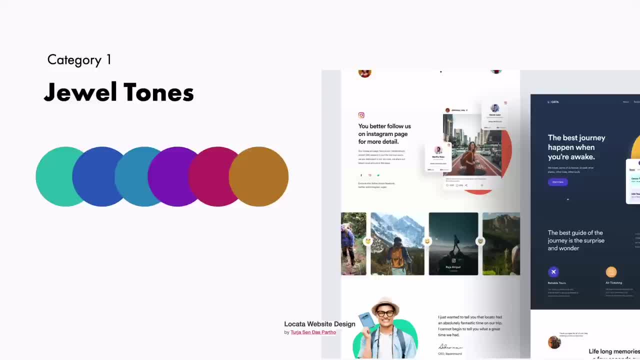 ruby red, amethyst, purple, citrine, yellow and emerald green. Think of the deep richness of a ruby red necklace or a royal purple crown. These colors are regal, deep and impart a sense of luxury. I've discovered that the ideal saturation and brightness for creating jewel tone color. 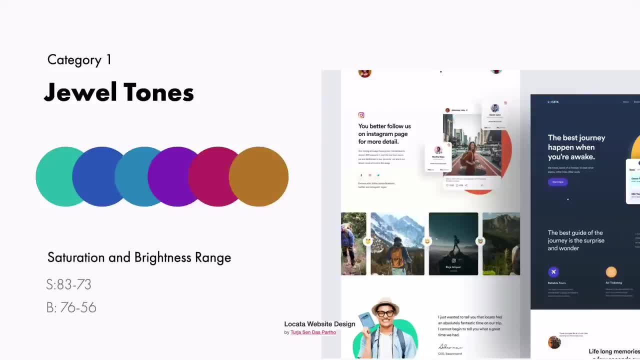 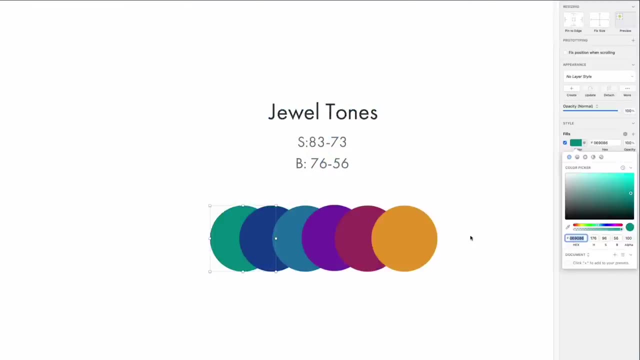 palettes lies within a saturation value range between 83 and 73 and a brightness value range between 76 and 56. So let's take a look at what that looks like inside of our design app. So, as I mentioned, the ideal range for jewel tones is any hue that has a saturation between 83. 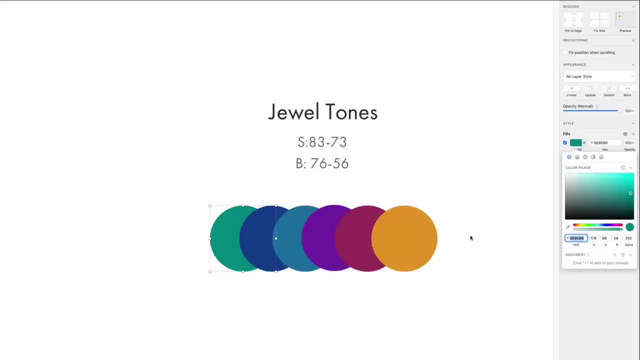 and 73 and a brightness value of anywhere between 76 and 56.. Let's see how we actually use this formula to create these jewel tone color palettes. First, let's start with a setting. We're going to start with a setting of 76 and 56.. So let's start with a setting of 76 and 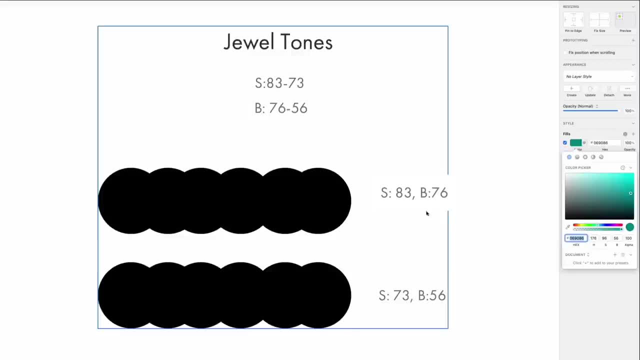 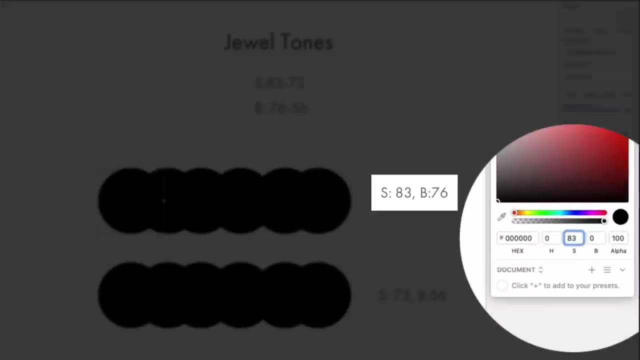 56. So here I have six circles that are all black. First thing we're going to do is take the first two values: the value of the highest saturation and the value of the highest brightness. So for our saturation, we're going to set this value to 83. And then for the brightness, 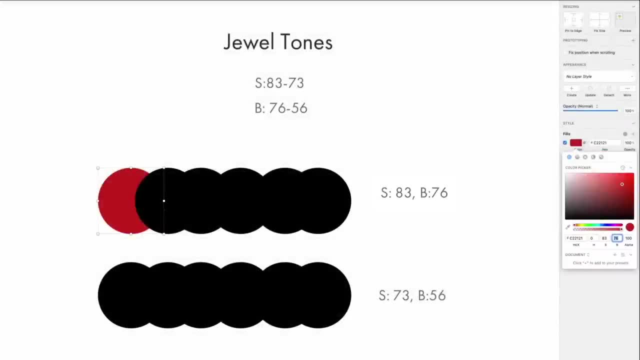 we're going to set it to 76.. What results is a beautiful, deep, rich ruby red color. For the rest of the swatches it's even easier because all we have to do is select the next swatch, copy the previous color and then, without touching the saturation or brightness. 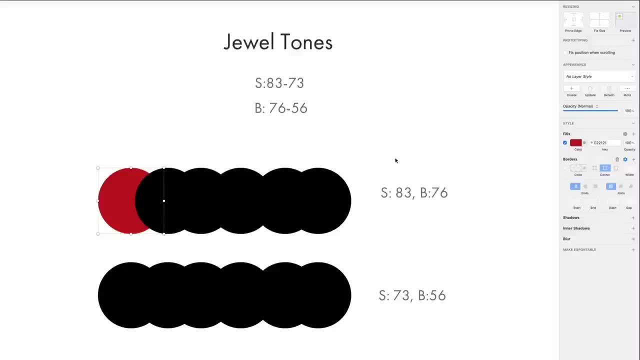 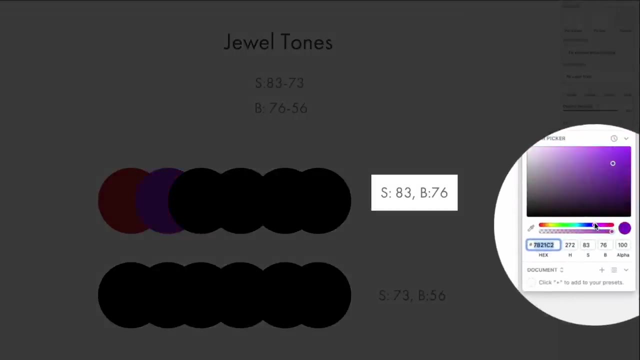 we're just going to slide the hue into a different color. So I select the next swatch, I match the fill color of the first one And then, without touching the saturation or brightness, I'm going to grab my color slider and just change the hue. 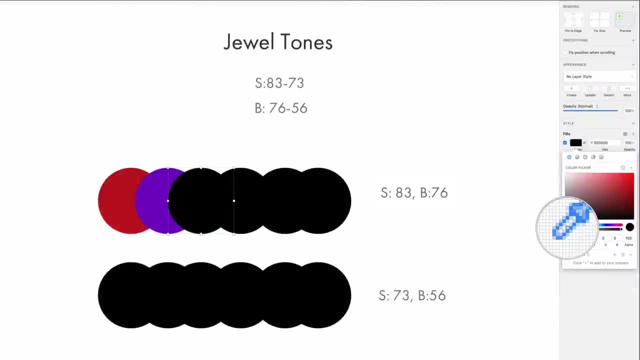 And then we continue to do that for every single swatch. Select the previous color, Then slide the slider And voila, you have a perfectly balanced dual tone color palette. With this color palette, every single one of these colors are going to be in the same color palette. So we're going to 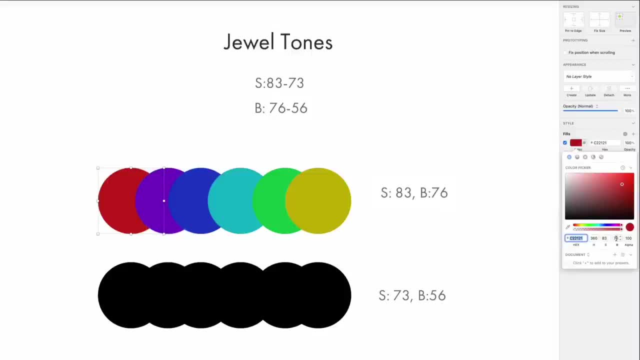 set the saturation to 83. And then we're going to set the brightness to 76. The only thing that's changed is the hue or the color. So again we have a safe range in which we can have varying tones and tints of our jewel tones. So let's try the other end of the saturation and brightness. 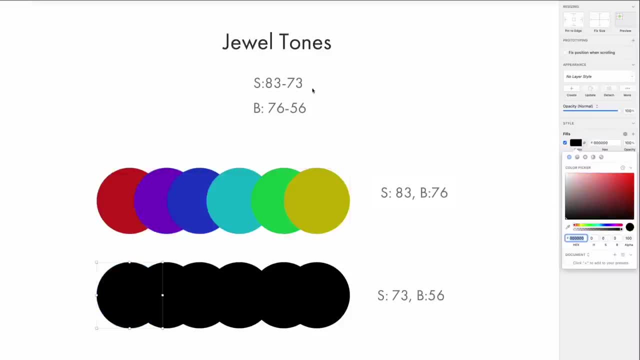 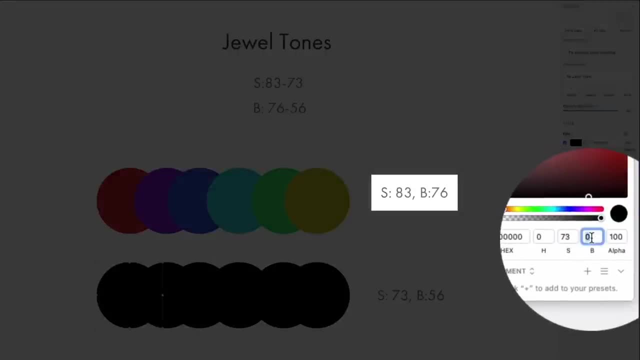 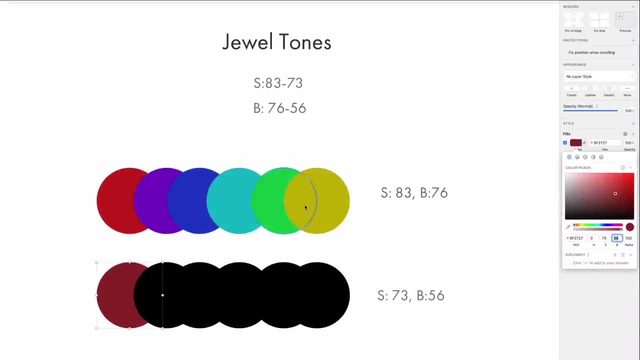 values. Starting with the first one, we're going to make our saturation 73. And then we're going to make our saturation 73. And then we're going to set the saturation to 83. And then we're going to make the brightness 56. So you can see that this results in a darker version of the colors that we. 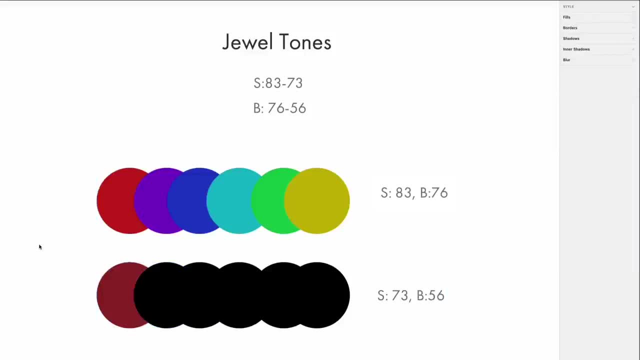 have in the previous palette. And then we follow the same technique of selecting the next swatch, copying the color from the previous swatch and then, without touching the saturation or brightness, just dragging the hue slider over, And then continue doing that for the rest. 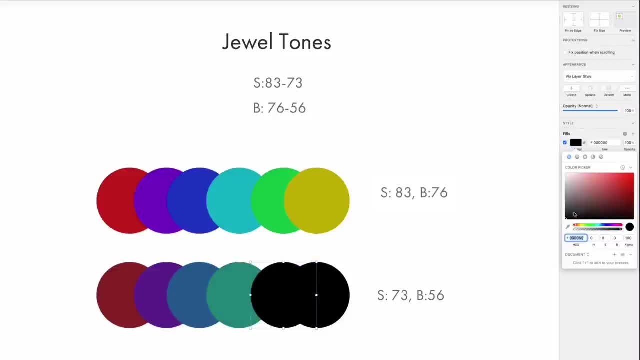 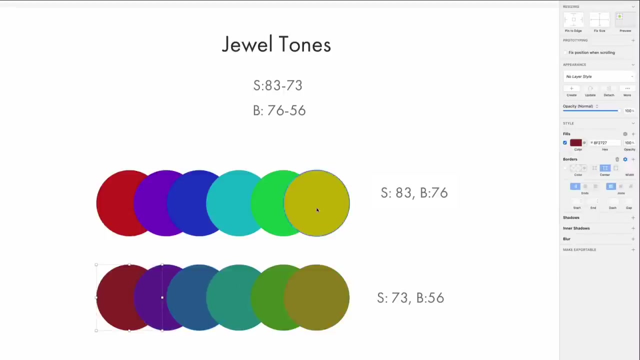 And now we have six more colors in our color palette, each of these with a saturation of 73 and a brightness of 56. And again, the only thing that we've changed is the hue. So within this range, you have the ability to choose other saturation and brightness values. 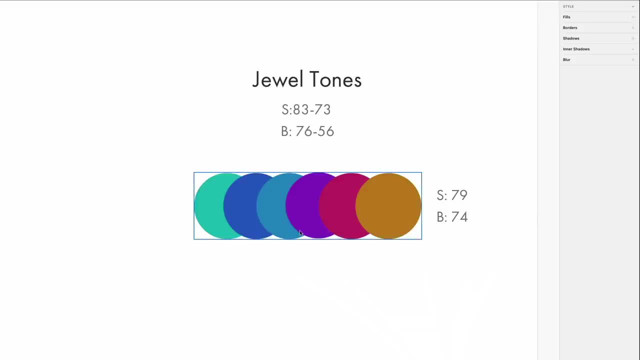 with this color palette, I'm somewhere in between the safe range of the saturation and brightness levels. each one of these swatches has a saturation of 79 and a brightness value of 74, and we know that we're still in the jewel tone range because 79 is in between 83 and 73 and the brightness of 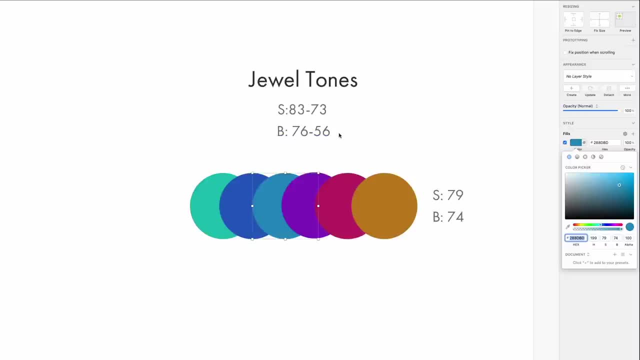 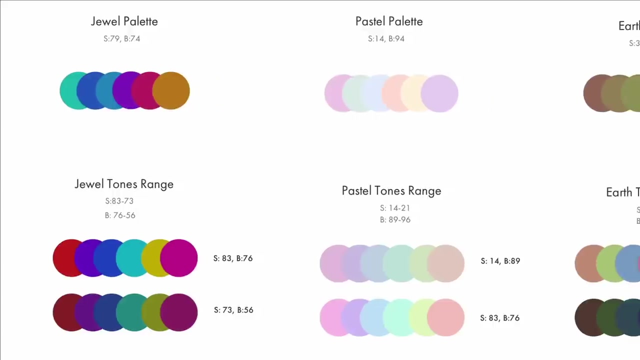 74 is still within the range of 76 to 56. so as long as you keep your saturation and brightness within these ranges and you only change the hue slider, you will still end up with a beautiful color palette that is jewel toned. this technique can be applied to every single one of the color. 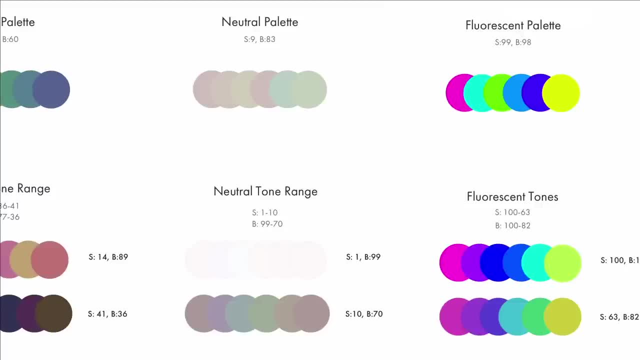 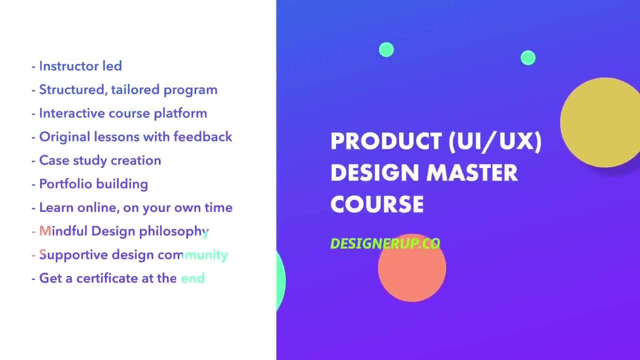 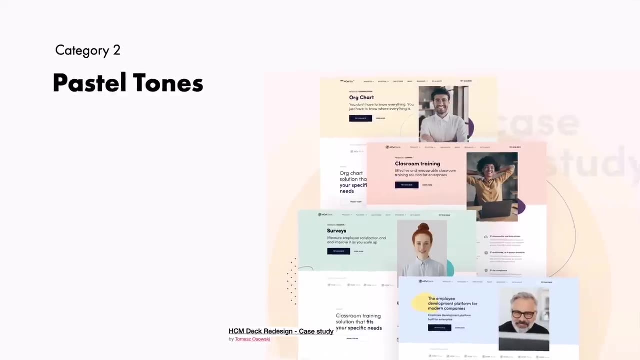 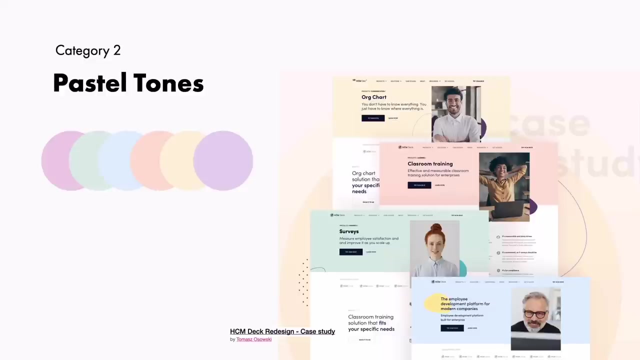 categories. so if you're interested in seeing these and more color formulas and color palettes, you should definitely come and have a look at our product design master course, where I dive even deeper into color harmony, color theory and color formulas. so the next category is pastel tones. these belong to a pale family of colors: pink, mauve and baby blue. 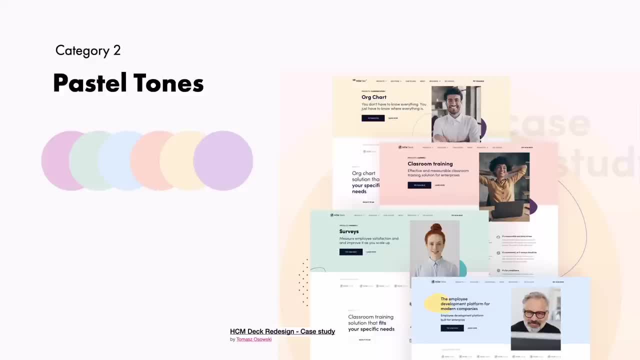 are commonly used pastel colors, as well as mint, peach, periwinkle and lavender. the colors of this family are usually described as soothing. we create these colors by reducing the saturation and adjusting the tone tint, or dragging our color pickers into the white area, the ideal saturation range for pastel tones. 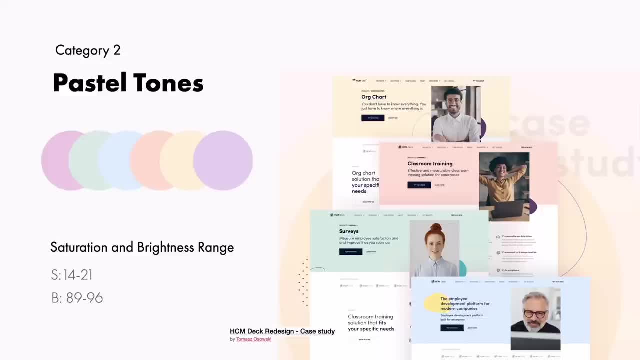 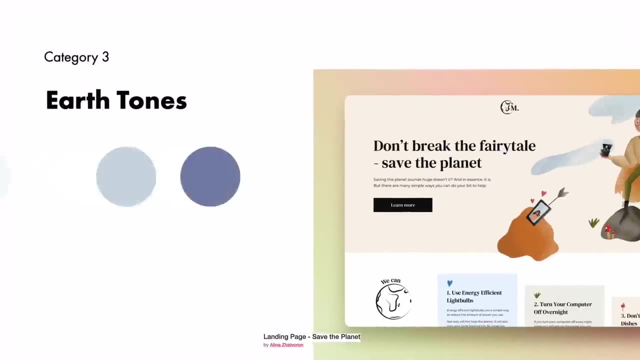 is between 14 and 21 and the brightness range between 89 and 96. category 3 is earth tones. these are colors commonly found in nature. many earth tones originate from clay pigments like umber, ochre and silver, and they are often used to create the color that we want for our colors. so 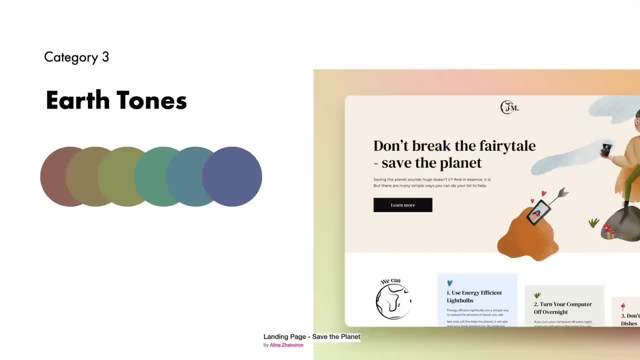 these colors are commonly found in nature. many earth tones originate from clay pigments like umber, ochre and sienna. they can be created by combining a pure hue with white, black or gray. these are considered, in the more broad sense, neutral colors. they are influenced by the tones of trees, forests, seas and 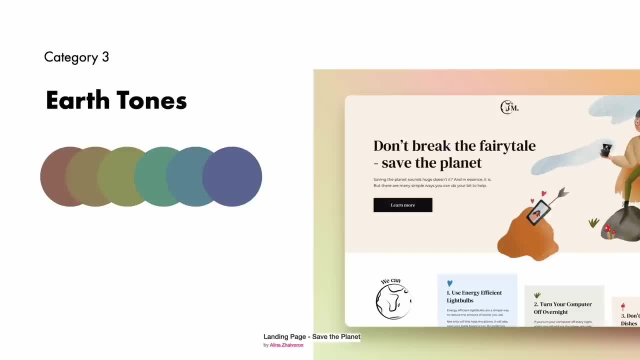 sky and are muted and flat to emulate natural colors. we create earth tones by increasing saturation and adjusting the tone or dragging our color pickers into gray. the ideal saturation range, saturation and brightness range for creating earth tones is a saturation between 36 and 46 and a. 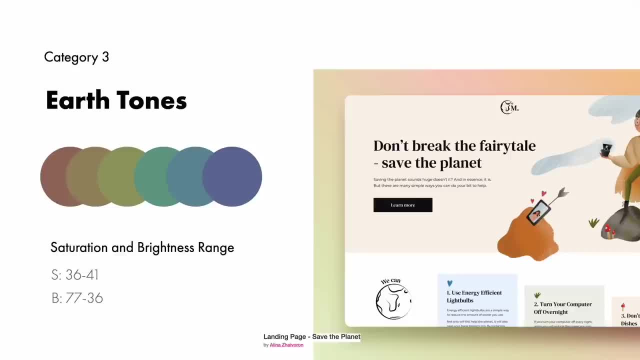 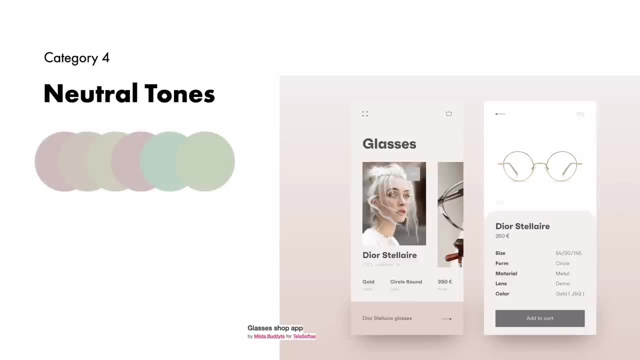 brightness between 77 and 36. category 4: neutral tones. pure neutral tones include black, white, beige and alpha gray is, while near neutral tones include browns, tan and darker colors. these are created by desaturating our colors. they pair with a gray and blue color combination using our medium colors. braveryjug has many more gauges, so this in addition. 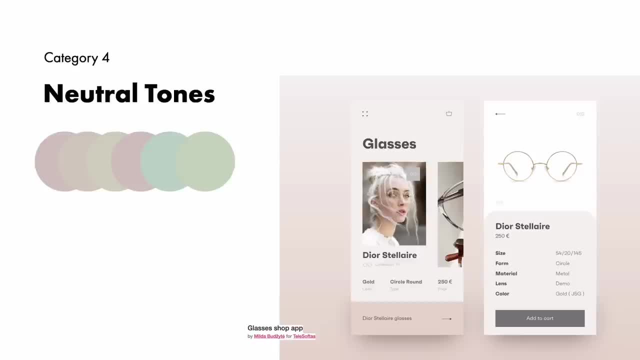 to fluor medallion. umber large, palver, Мосkv της are spotted in similar colors as black, hair, gray, real. these colors along here appear on a putty palette to fit various colors in contrast to pink and launch very skinny shades. but they're more than that of cool shades. now, colors with integrand votes can be. 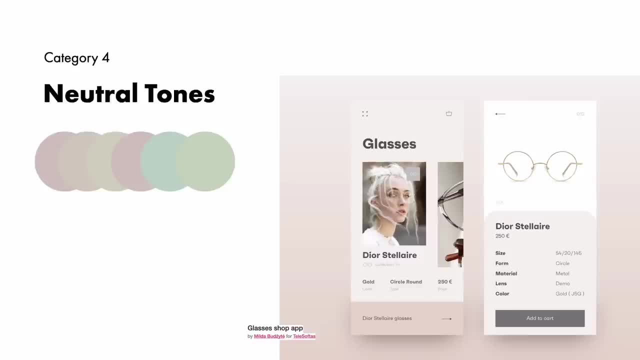 Pair well with any of the other categories of colors. to create balance, We create neutrals by decreasing saturation and adjusting the tone, tint and shade, meaning dragging our color pickers closer to the white-gray-black side of the color picker. The ideal saturation and brightness range to create neutral tones is a saturation between: 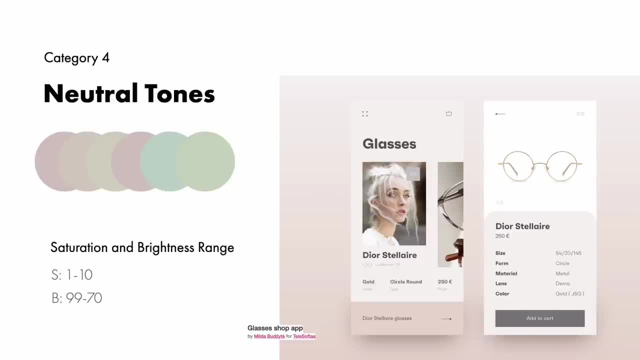 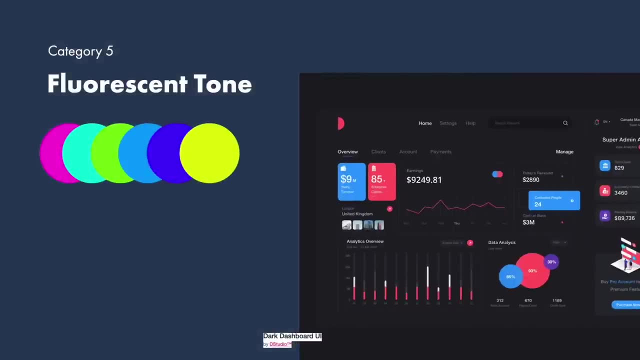 1 and 10, and a brightness between 99 and 70.. Category 5, Fluorescent Tones, sometimes called neon tones. Fluorescence is a result of photoluminescence. Phosphorescent color emits light when excited by visible or ultraviolet light. 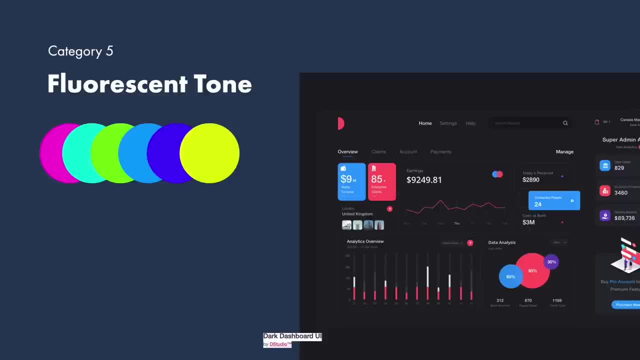 In the physical world, this is created by neon tubing in which light is projected through, or ultraviolet reactant paint colors, But in the digital world we can get a similar effect by applying very bright and highly saturated colors to our designs. 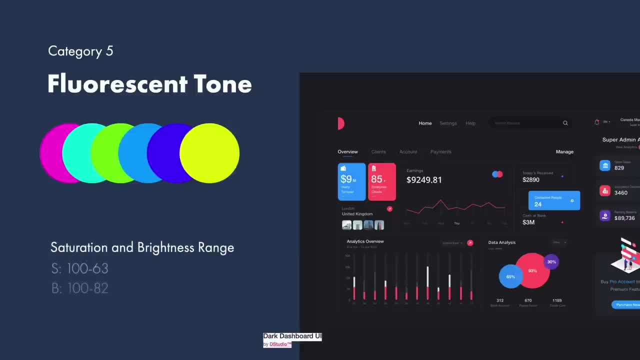 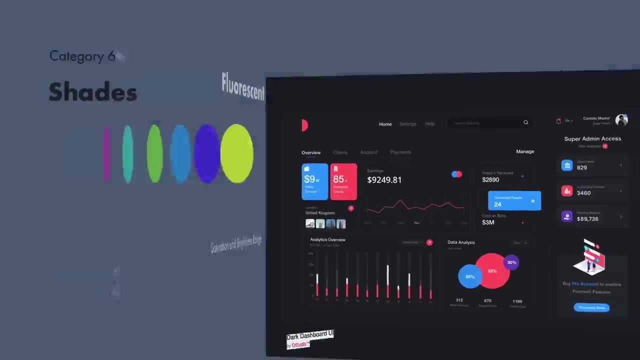 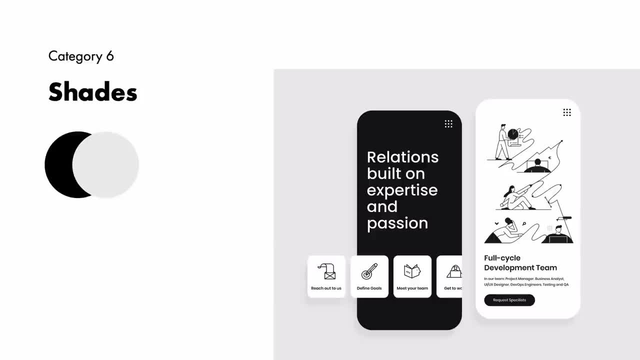 The two main shades are black and white, which are not normally considered colors, but rather the absence of light or dark, or the addition of pure shade or pure tint. Other shades include all varying degrees of gray. The ideal saturation and brightness range to create shades are a saturation between: 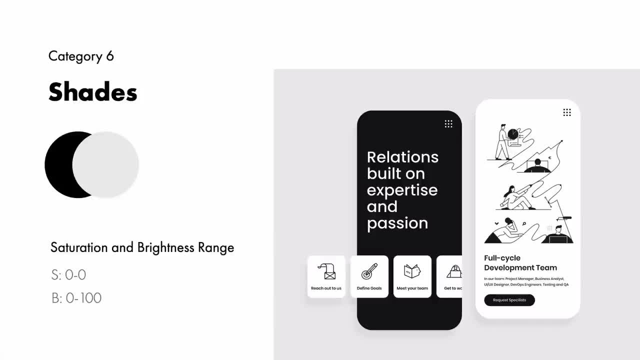 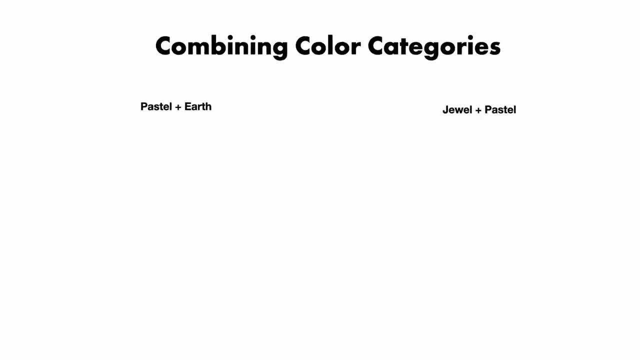 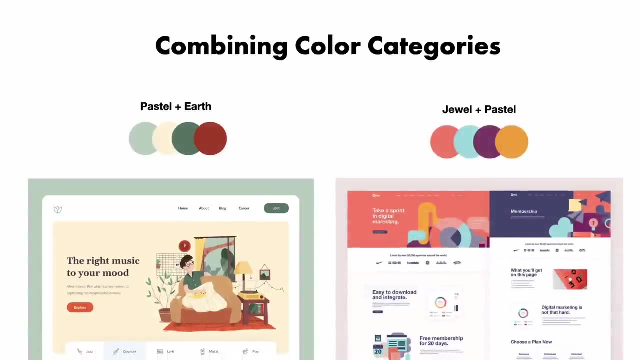 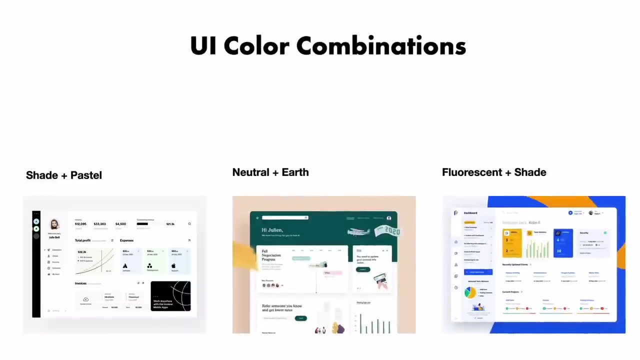 0 and 0, and a brightness between 0 and 100.. Combining color categories. You can also combine these different color categories, such as pastel plus earth tones or jewel plus pastel tones. The best user interface designs use a combination of one of the main color categories, along with. 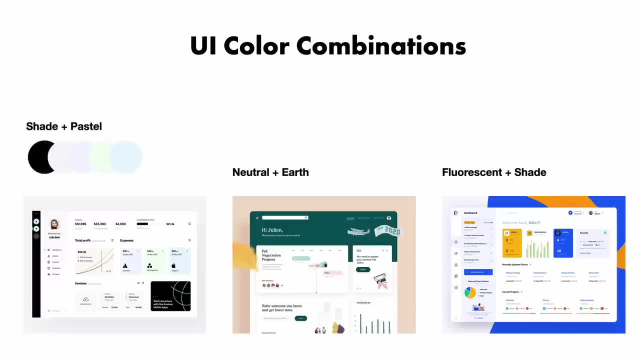 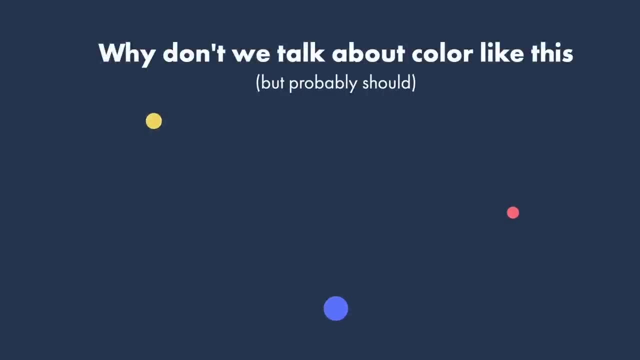 neutrals and shades. Shades plus pastels are commonly used, Neutrals and earth tones are seen a lot, And fluorescents and shades, whether on dark design or light design, are very common. So why don't we talk about color like this? Well, as digital designers, we tend to avoid.